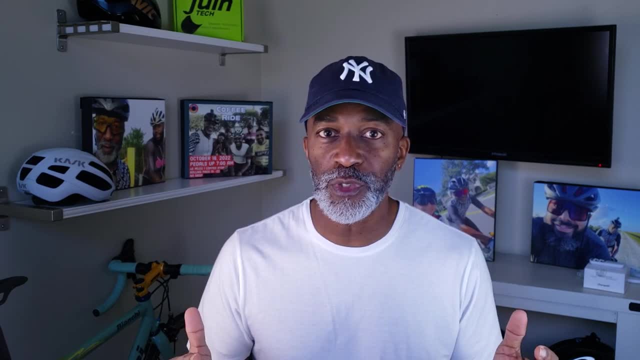 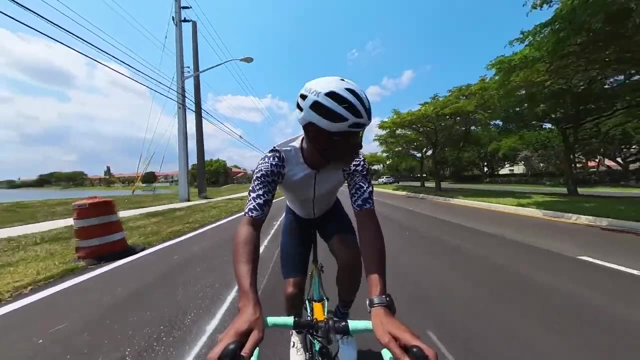 about how to look back effectively. To me, there's no substitute for using your eyeballs to get a full picture of what's going on behind you. So, yeah, you can do both, All right, so let's jump into this. What I'm going to actually talk to you about today is I'm going to talk to you about things that you need to check on your bike before every single ride. I'm also going to talk to you about things that you should check every one to two weeks, And then I'll talk to you about the things that you should check on your bike at least monthly, just to make sure that you're. 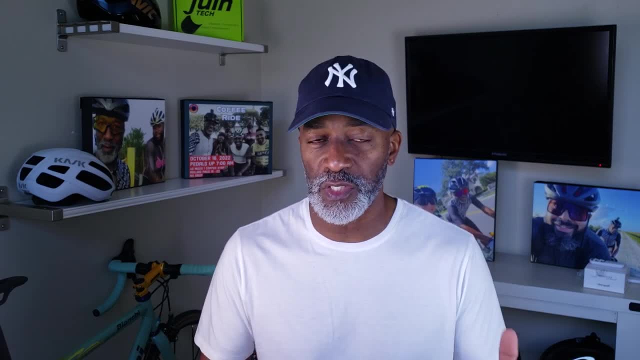 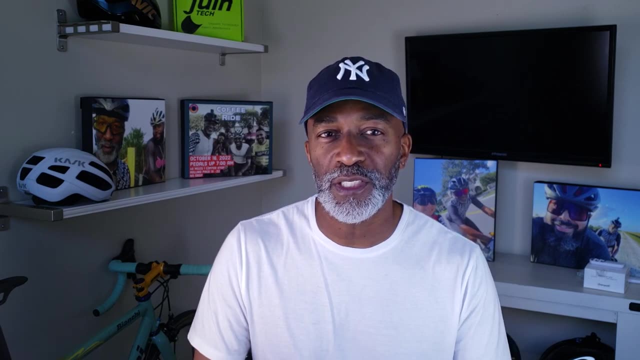 equipment is tip top. It doesn't mean that you have to fix this stuff, but I think it's important for you to know what's going on with your machine. So we're going to talk about how to identify those potential problem areas. Now, in my defense, on the ride up to Central Florida- it's not that I 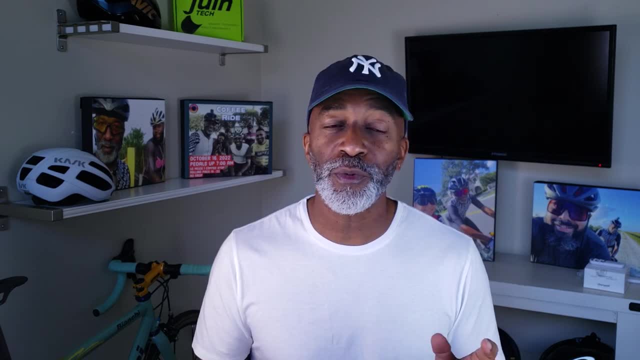 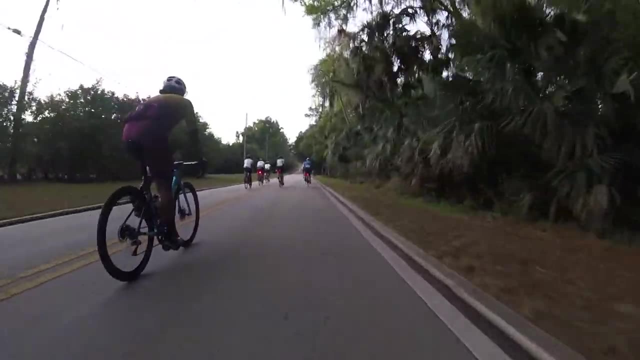 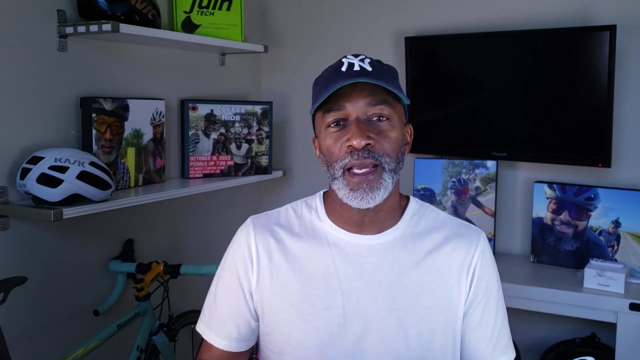 neglected my basic bike maintenance. it's that my rear brake- the spring on my direct mount brake- was actually malfunctioning to the point where, once I applied my rear brake aggressively, the spring did not return The brake. it ended up in a cockeyed position and I ended up having a rub master more than anything. 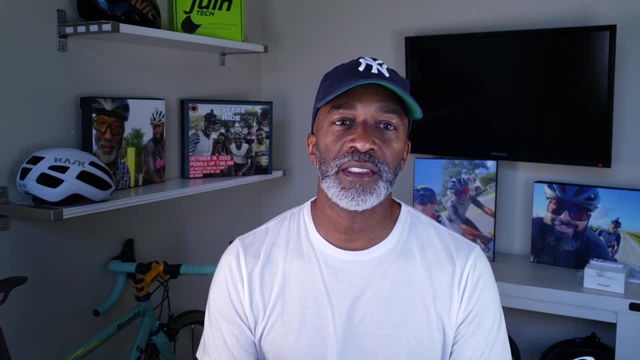 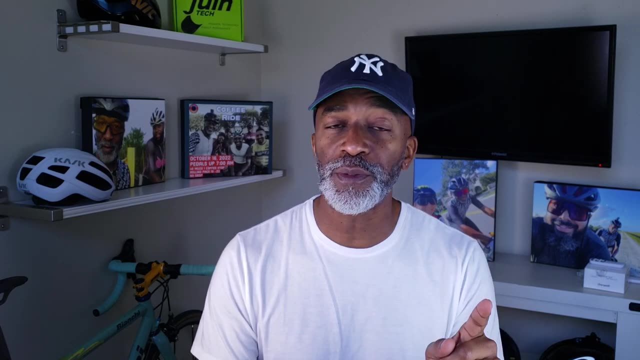 else. So we're going to begin this by talking about the things that you need to check on your bike before every single ride. You need to make sure that your tires are tip top, and you also need to make sure that your chain is tip top. So let's talk about how we do that properly. We begin with. 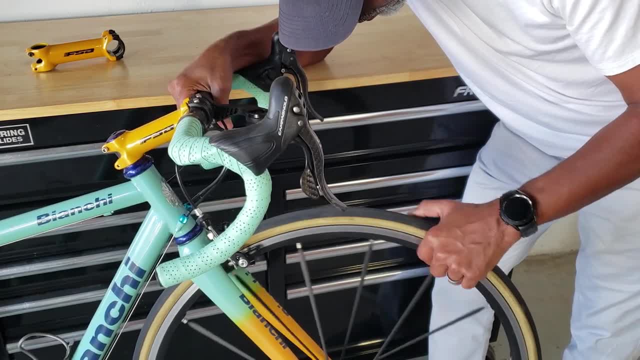 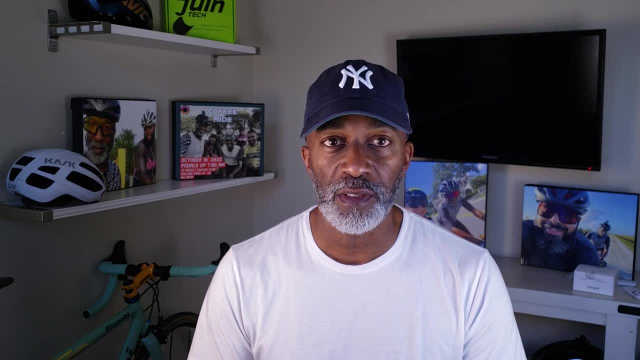 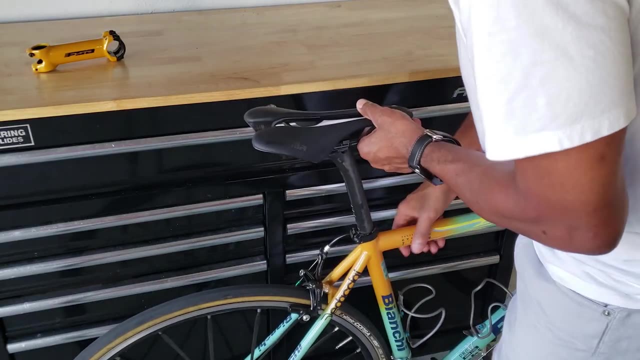 a visual inspection of the tires, and your tire inspection is probably best performed the night before the race. What you want to do is you want to check for rips, gouges, obviously, anything that's poking out or protruding out of your tires, slashes, thread, wire that's showing anything. 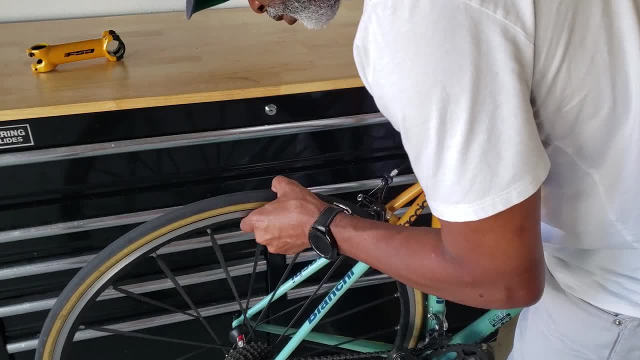 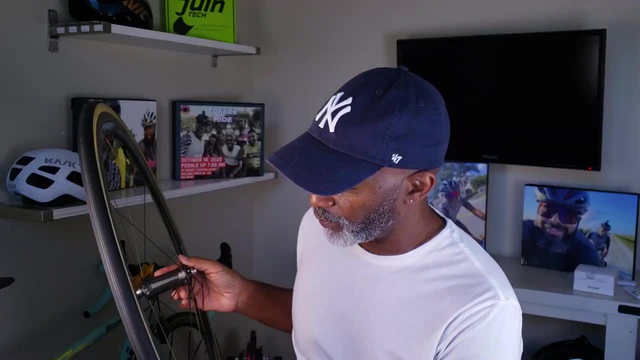 that's like man, my tire is really worn. You also want to look for uneven wear of the surface of your tires, much like you would look at the alignment of your car. If you're running tubeless, you want to make sure that you don't have any sealant or anything seeping out, And if you're running a? 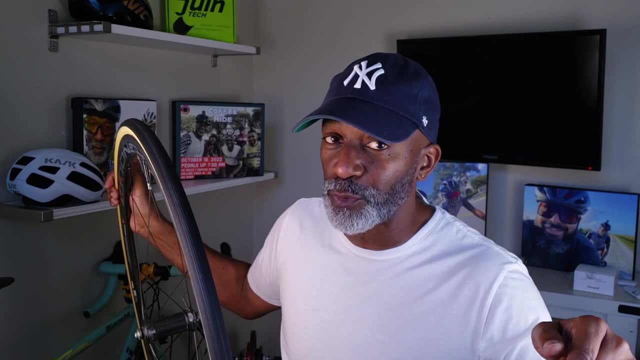 flat tire. you want to make sure that you don't have any sealant or anything seeping out. You want to make sure that you don't have any sealant or anything seeping out And obviously we want to make sure that we check the tire pressure right before the ride. make sure that our tires are. 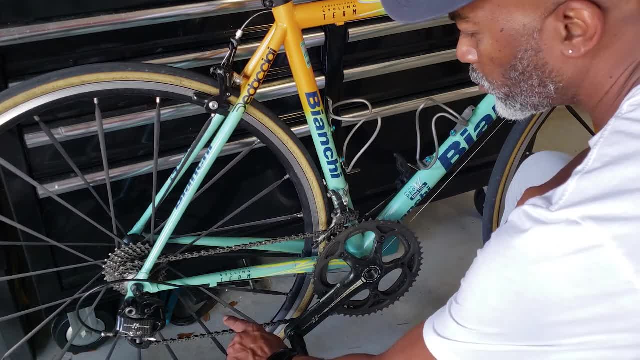 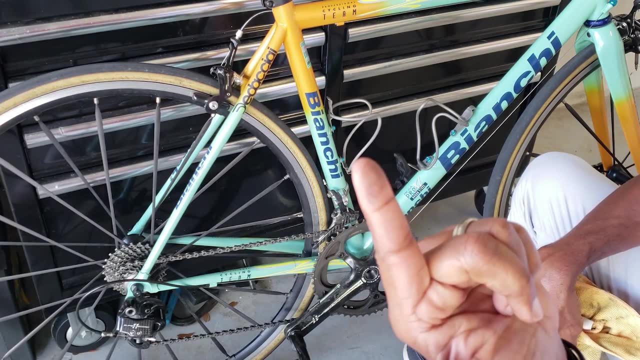 holding air. Next, we've got to check the health of our chain And, again, this is one of those things that you're going to do before every ride. I actually did a video on how to clean and lube your chain. I'll post a link to that in the description. I just run my fingers along the 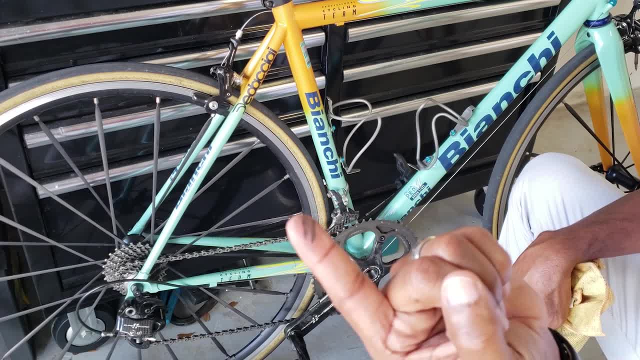 inside of the chain just to check the viscosity of the lube that's on there, Make sure that it's not too dry, not too gummy, and also want to make sure that it's not too watery to where it's not. 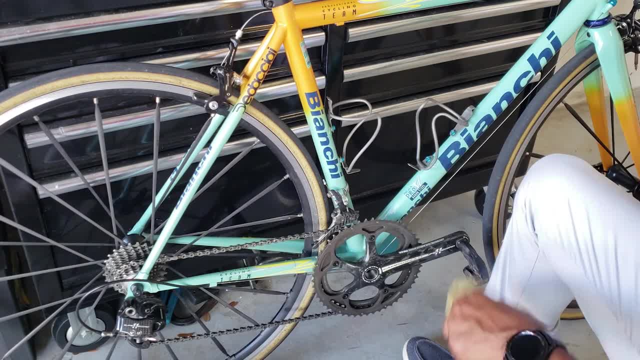 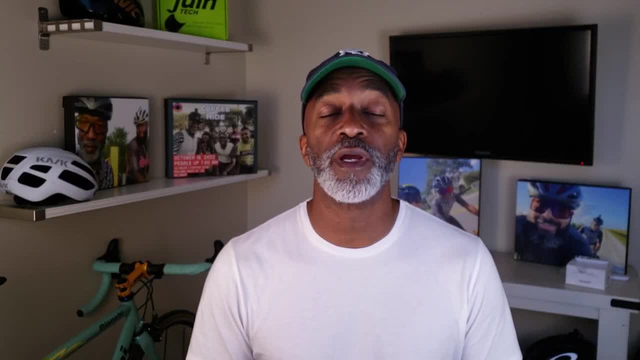 doing the job that it's designed to do, which is to keep the chain properly lubricated so that my drivetrain is working efficiently. And that brings us to the third and final check that you perform before every single ride, And that's just to make sure that your brakes are grabbing and releasing. 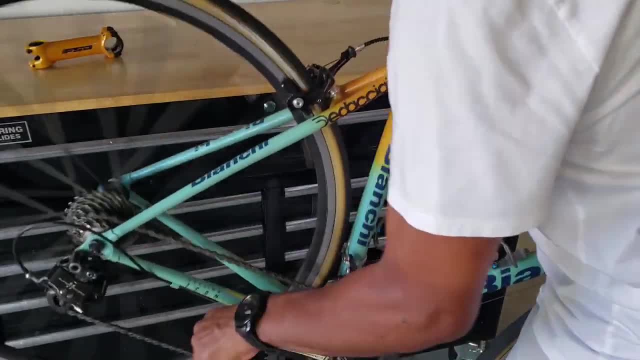 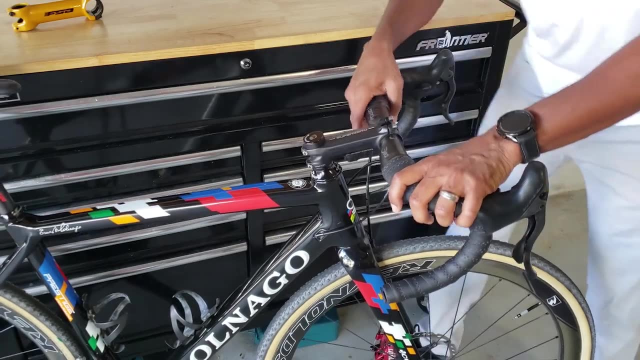 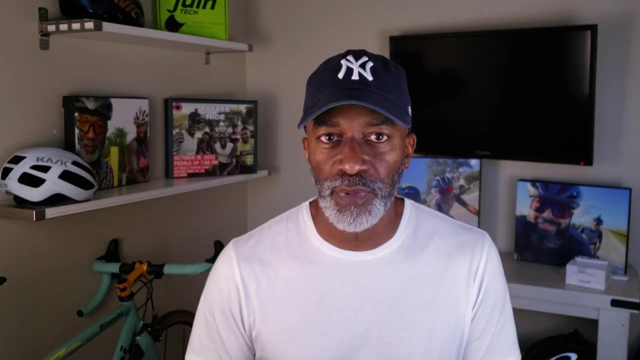 properly. I know ironic, isn't it. Simply spin your wheel, apply the brakes and spin the wheel again. It's that simple. And if you have any situation where you have sticky brakes, you have a bent rotor or anything like that, those things will present themselves with that simple. 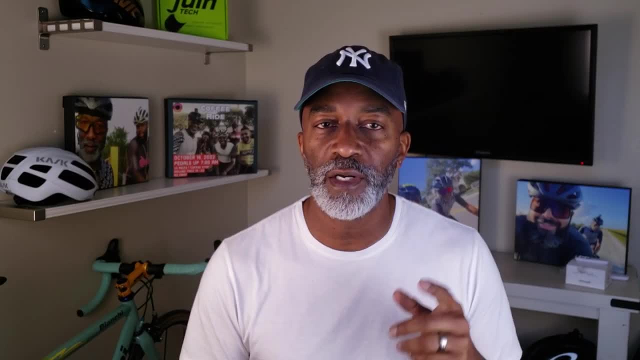 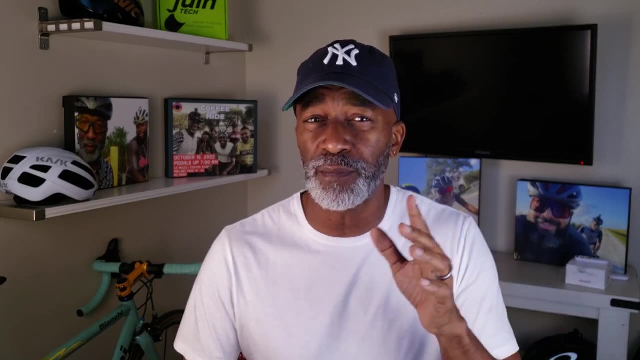 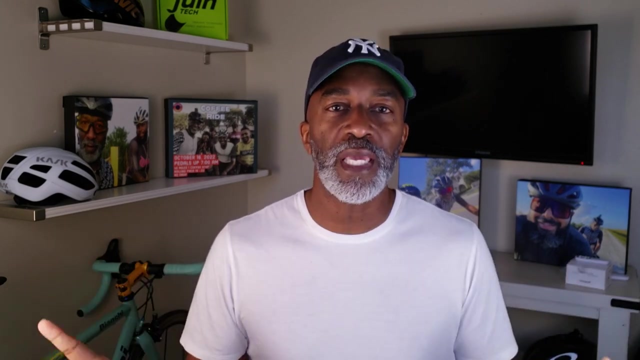 inspection. Now we come to checks that we have to perform every one to two weeks. Now, if you're putting in like 250, 300 plus miles every week, or even more than that, you need to be doing this every week. If you're like me, where you're barely getting 70 to 100 miles in a week, you're okay. 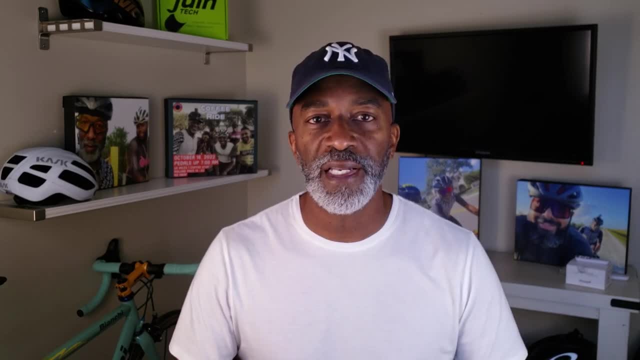 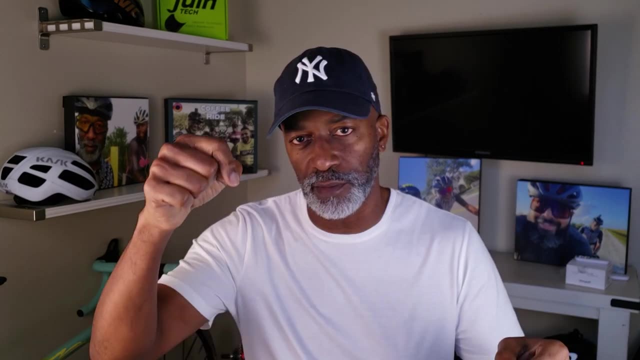 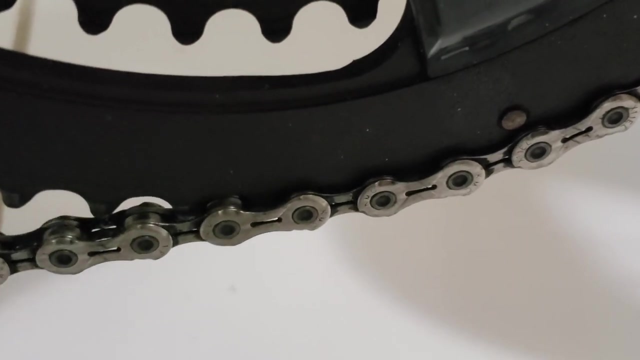 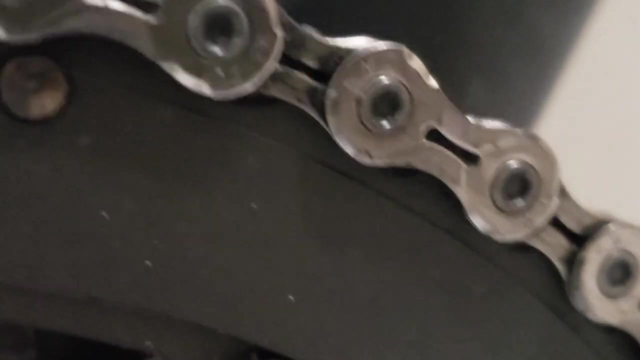 with it too. You can even probably stretch it out to about every three weeks. And that's to check to make sure that your chain is seating properly on the chain ring. You'll actually hear it, if it's not, when you're riding and when you're shifting gears. And, lastly, these are the safety and 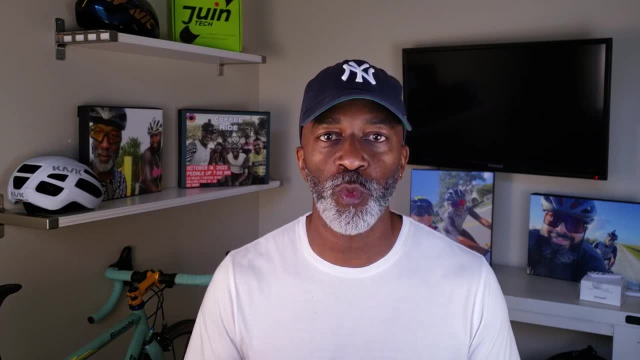 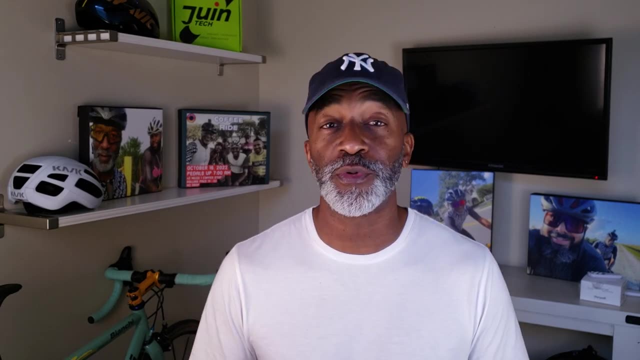 performance checks that you've got to be on top of at least once a month. And again, if you're riding on a regular schedule- and to me that would be like you're putting in about a hundred and 25 to about 300 miles a week- you need to be performing these checks every month, Okay, First, 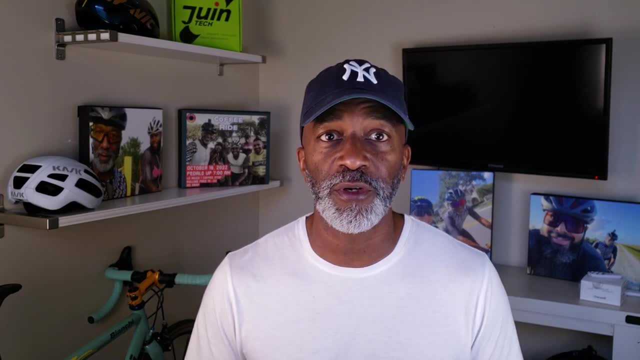 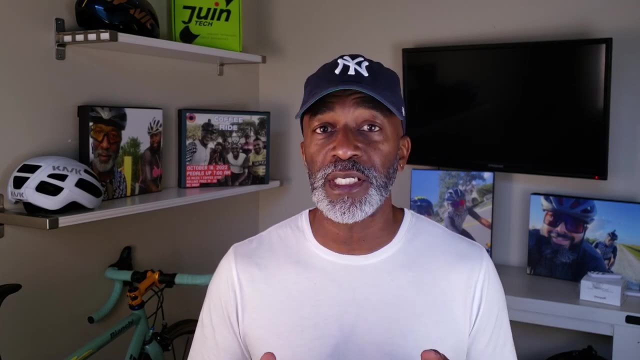 one being checking the health and the adjustment of your headset bearing. That can not only be a performance issue but also a safety issue. Also, your wheel bearings- huge potential safety issue. And lastly, we're going to talk about how to check your bottom bracket bearings Now in these: 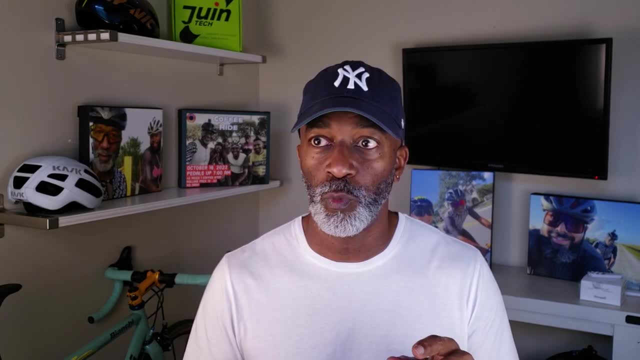 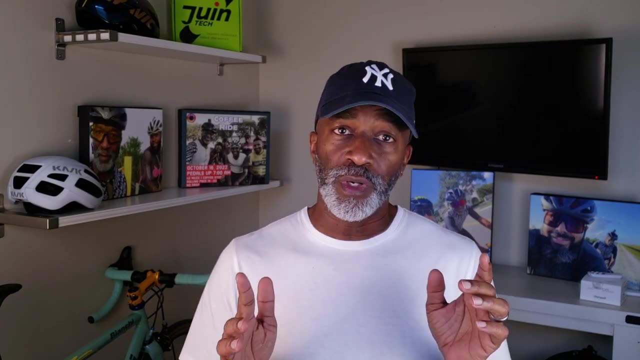 it's not so much about whether or not your bearings are worn out or not. These checks are to make sure that you're not getting any of that. So if you're riding on a regular schedule, you're going to want to make sure that the preload on the bearings are properly set up. We're going. 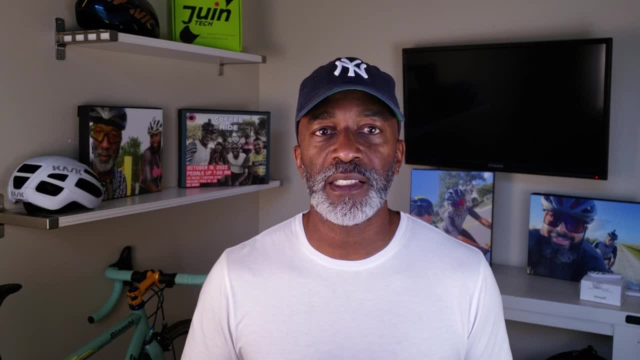 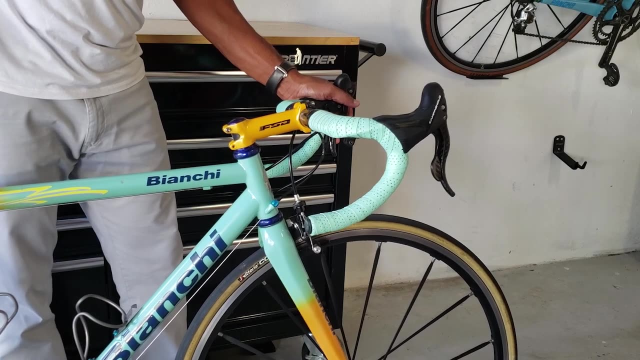 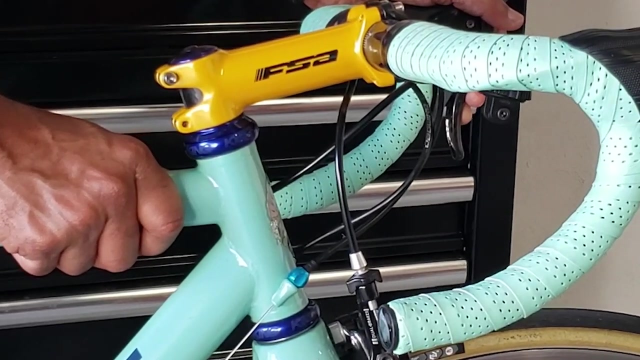 to begin with the headset bearings. Simply make sure that your bike is on a flat, stable surface. then apply the front brake And while the brake is applied, rock the bike back and forth. If your headset bearings are not properly adjusted, you will see the top cap for your headsets moving. 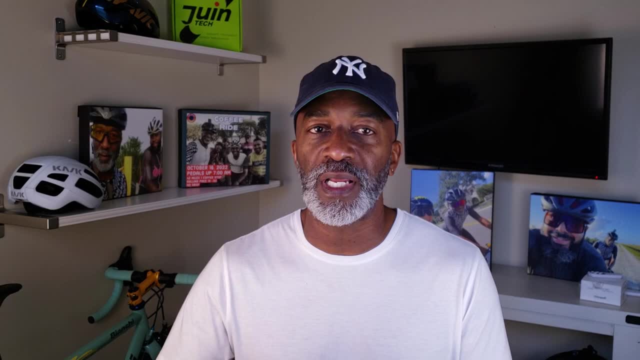 visually moving or you'll hear some sound coming from there. Now you will get a little bit of movement. You're going to want to make sure that you're not getting any of that. So if you're not getting any of that movement from your bike, that's to be expected, because you're applying 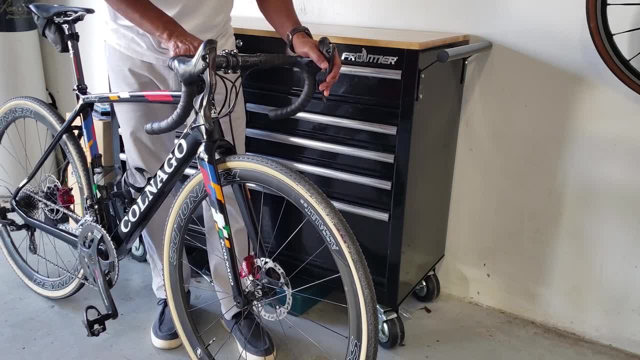 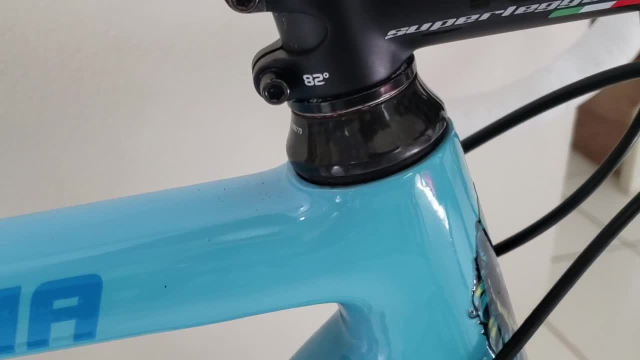 force to it, but you should not get a click, click, click or where you can actually visually see the top cap for your headset moving back and forth. And if you're in a situation where you're getting significant movement from your headset bearing or your top cap, it may not mean that. 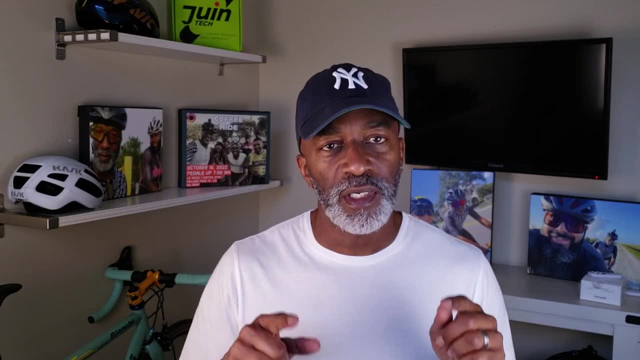 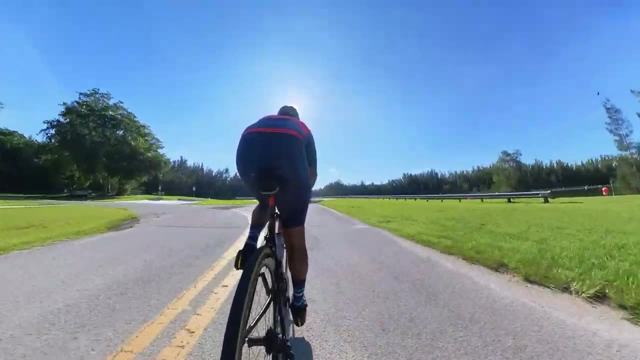 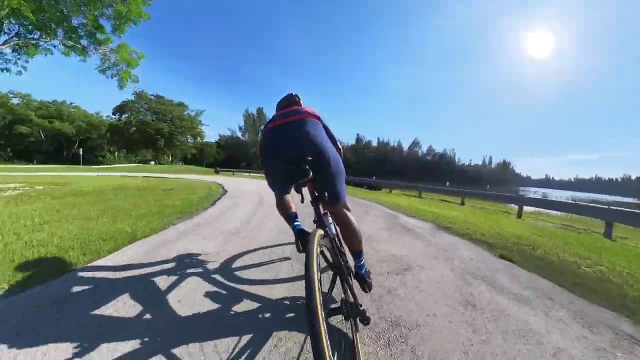 the bearings are worn out. It just means that the preload needs to be properly adjusted. Take that to your mechanic if you do not know exactly how to do that. Up next is checking our wheel bearings. Now your wheels really take a beating on rides, because not only are they spinning, going forward, 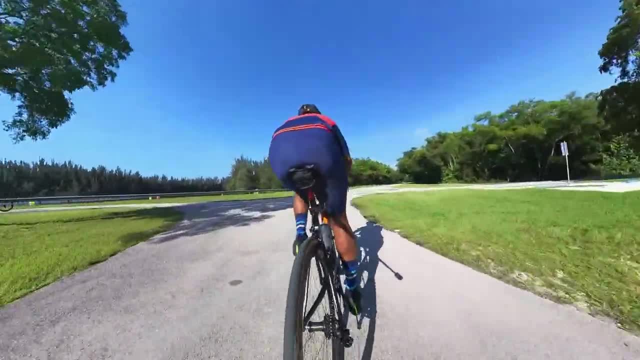 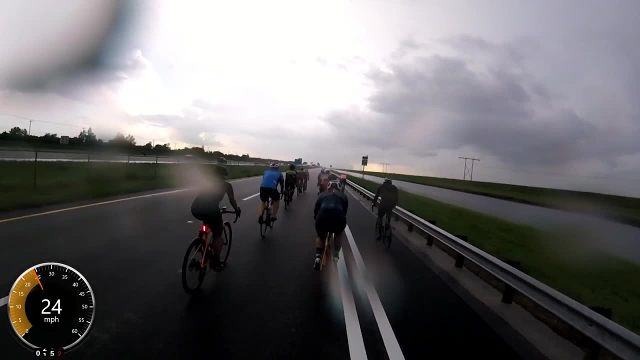 but they're getting a lot of load put through them. Every time you go through a corner or you hit a bump or something like that. they're basically getting abused, Not to mention if you're riding in inclement weather, where water is getting in there. But the way that you check. 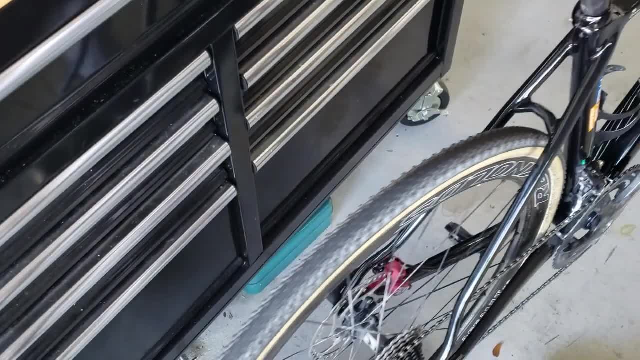 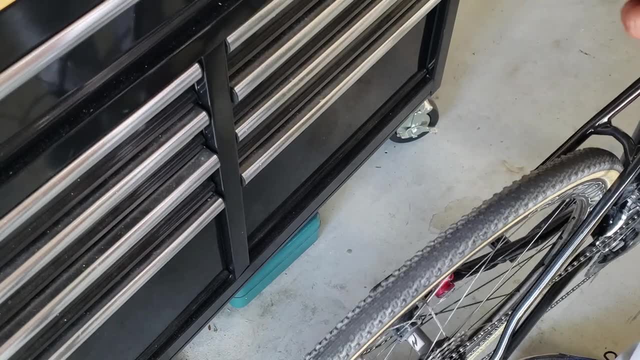 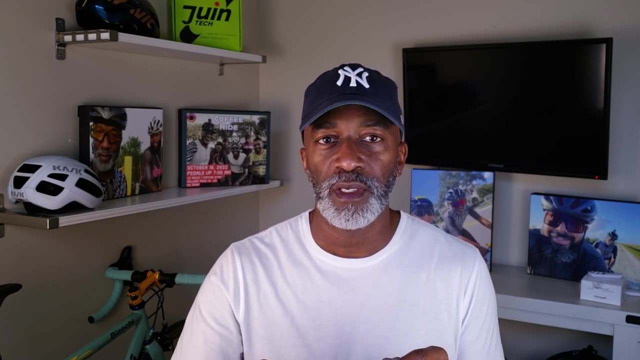 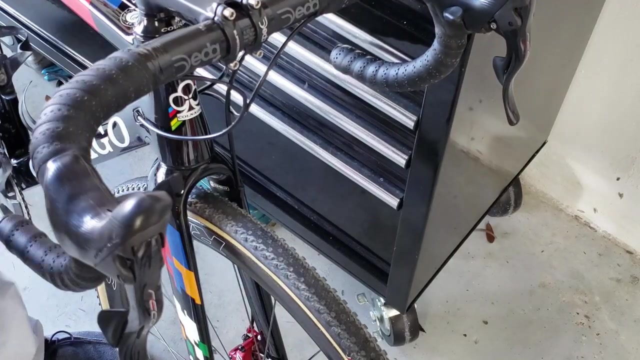 the preload or the fitness is to simply place your hand on the top of your wheel or the tire and simply rock it back and forth from side to side. If you're getting either one of those, it means either your bearings are completely shot, they're worn out, or it means that the preload in them was set so poorly that now you have 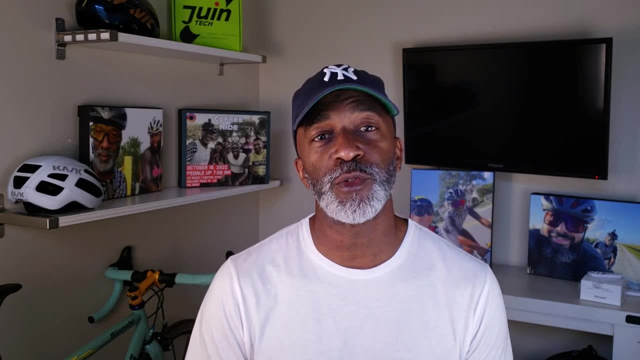 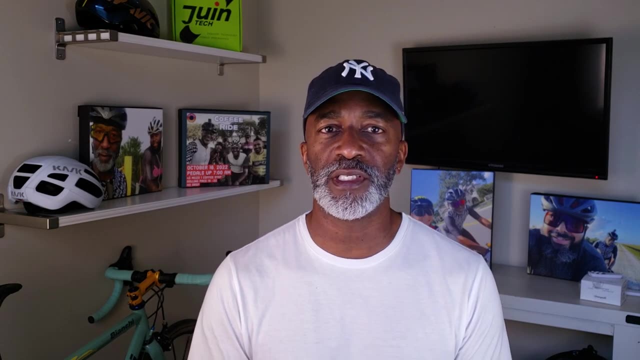 worn out bearings, So that's one that you definitely have to make sure that you take it to a competent mechanic right away to make sure that that gets serviced properly. Yeah, worn out bearings aren't just a safety issue, but they're also going to 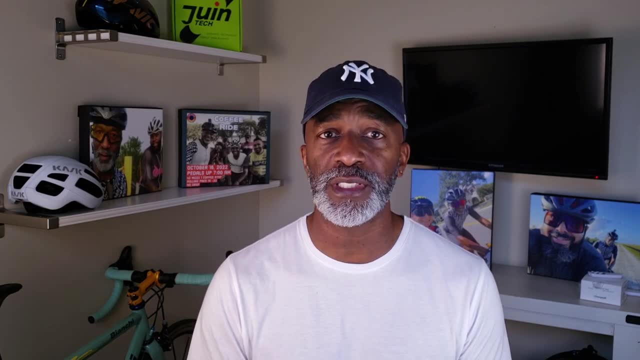 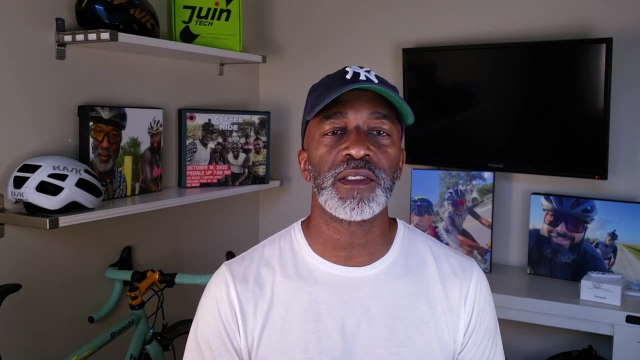 have a chance to get you in trouble. So if you're getting a little bit of movement, they're going to have a tremendous effect on the performance of your bike if that preload is not set right and if your bearings are worn out. And the last and final check that we do on a monthly basis with our bike is to make sure.